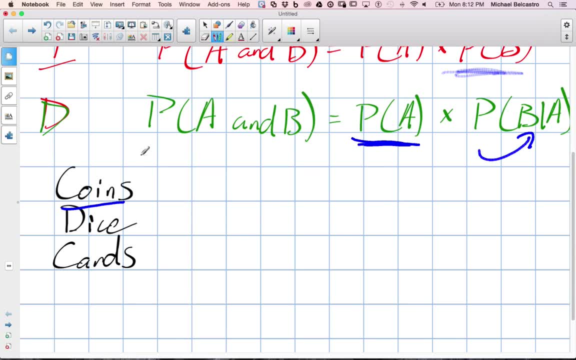 So we'll use kind of some classic examples. The first one we'll talk about is coins. Okay, a classic question might be flips. So what's the probability of A and B happening, The probability of getting three heads in a row? We know, on a coin you either get heads or tails, right, So you get one or the other. Well, in order to get a heads, okay, so you get. you know, if we made a factor tree, you have our heads, or probability tree heads and tails and they're 50% each, so you could say 0.5 and 0.5.. Okay, so once we get heads, does the probability of getting a heads the next time around change? 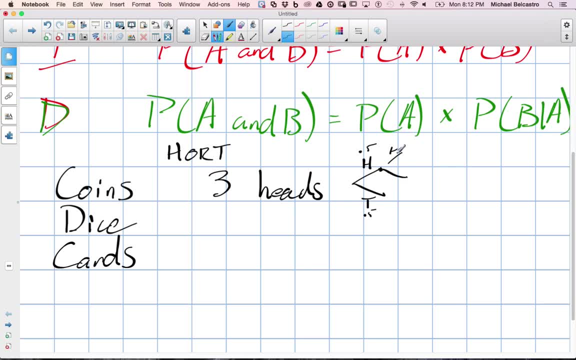 Is that? are we going to be less likely to get heads when we flip that same coin after No? No, it's going to be the exact same. So because it's going to be the exact same all the way through, I'll do it one more time: heads, and you get a 0.5 chance again. Does that make it an independent or a dependent event? 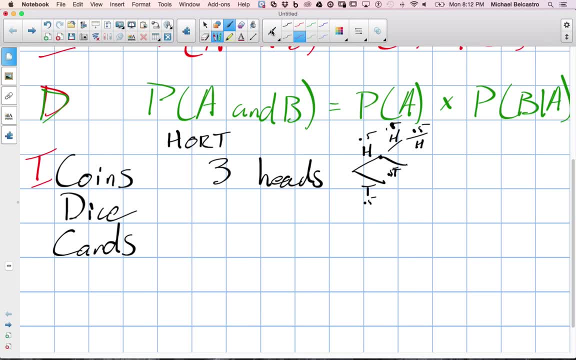 I'm going to say independent. That's right. It's independent because it doesn't matter what happened the flip before- right, It doesn't matter whatever happened the flip before. You still have the exact same probability moving forward when you flip the coin. 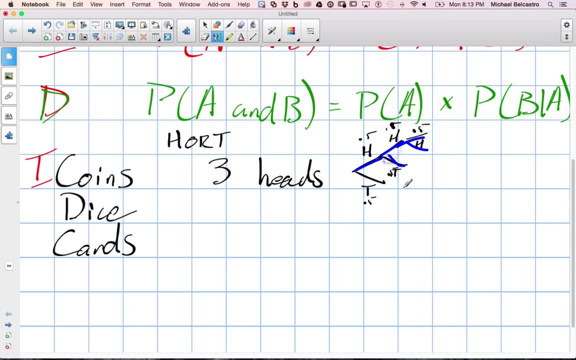 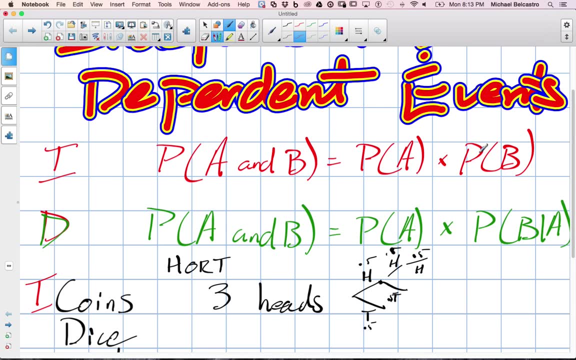 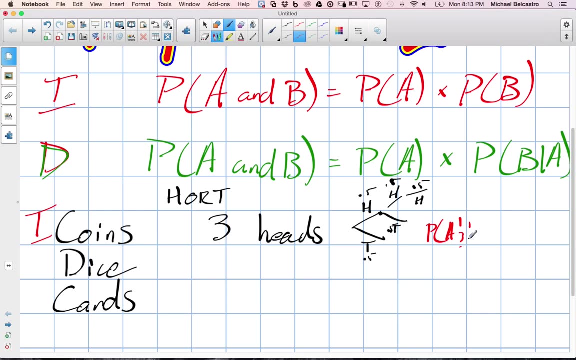 It's the same coin, a different coin, it doesn't really matter, The probability stays the same. Okay, so the probability of getting three heads- because we just discussed how it's a probability of event A times event B, and then we'll say event C- well, that would be, let's say, probability of A and B would be 0.5, or 50% times 0.5, times 0.5, so 0.5 cubed. 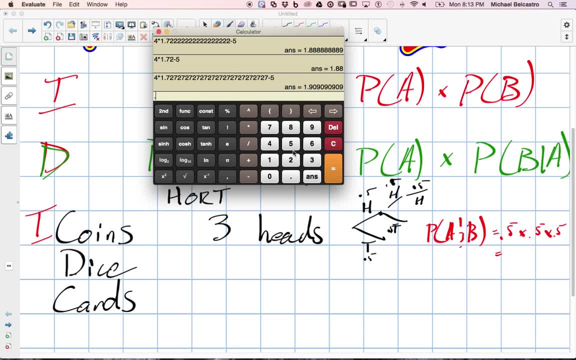 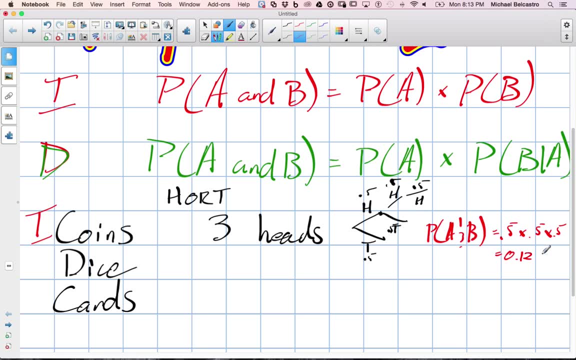 So in order to solve that, let's do 0.5 to the power of 3.. 0.5 to the power of 3,, 0.125, that's what I thought. So the probability of that event happening is 0.125, or 12.5%, getting three heads in a row. 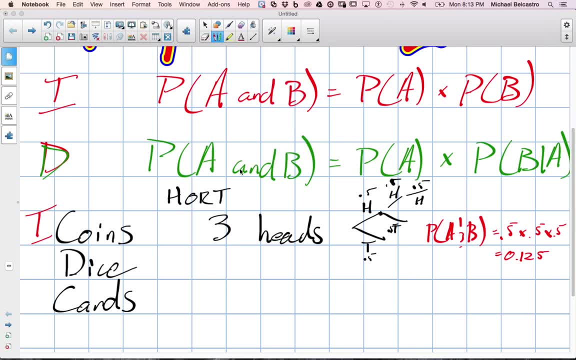 Okay, next thing: dice For rolling a die. what's the probability of getting? we'll say, three, threes. I don't know why it took me so long three, threes in a row. okay, so let's think about rolling a die. uh, what's the? 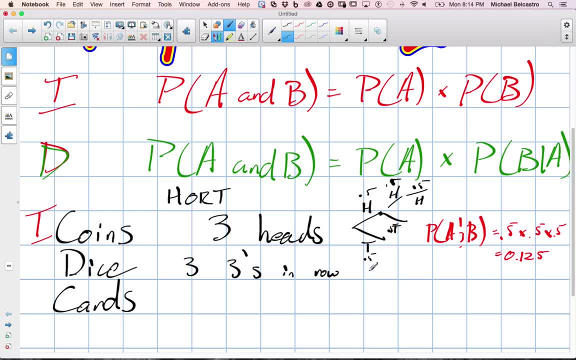 probability of getting a three. that's right. so to get a three, we have a one in six chance. okay, now, because we roll a three the first time, does that affect our probability of our second roll? does it change this probability? no, no. so what's the probability of getting a three again? 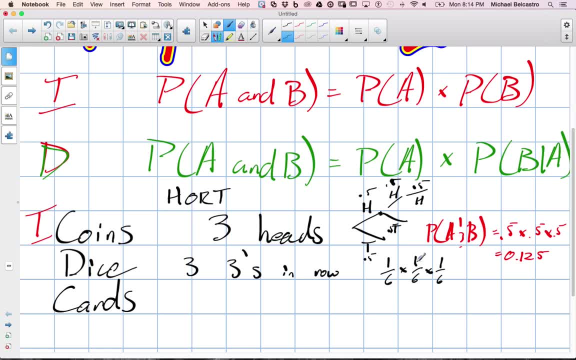 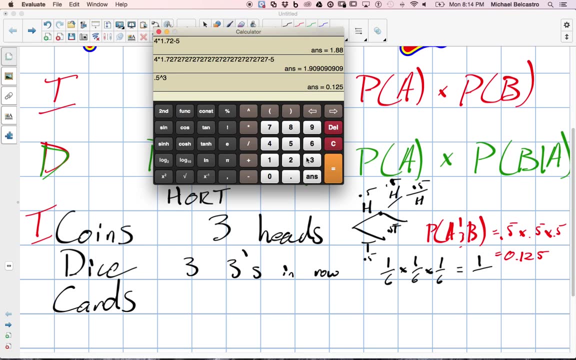 yep, and then that just keeps happening, okay, unless literally the sides of the dice are blowing up and we have less sides independent. they are very independent events, it does not matter what's happening. so we're looking at: uh, one over and what's six times 36. 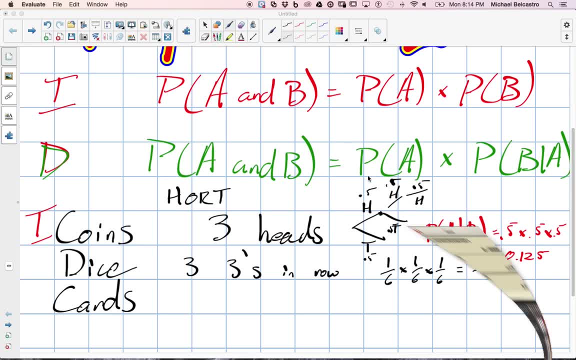 216. so one in 216. whatever that percentage is, would be the probability of getting three threes in a row, which means this is independent again. okay, let's talk about, um, getting three kings in a row. okay, from cards. okay, um, do you know how many kings are in a deck? 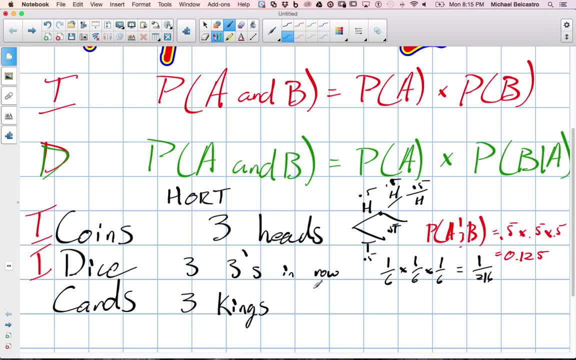 of cards, or there's four. and do you know how many cards are in a deck of cards? 52, yes, so we have a four and 52 chance of getting a king on our first one. okay, so once i draw the king out, how many kings are left in the deck? three, three, yeah. and let's say i drew a king the very first time. um, how many? 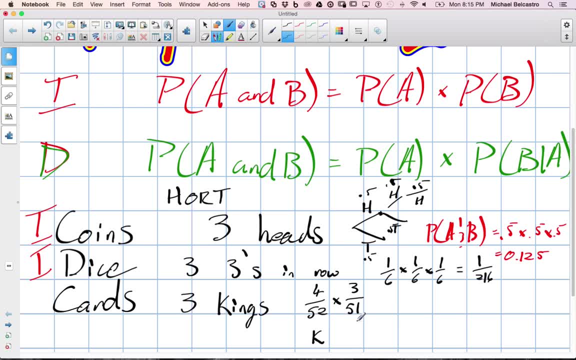 kings are left in the deck 51, 51. okay, so that's for drawing the next king. what about for the next king? how many kings are left in the deck two? two, how many cards are left? okay, has the probability of each event stayed the same? no, it's changed so which means what type of an event is this? 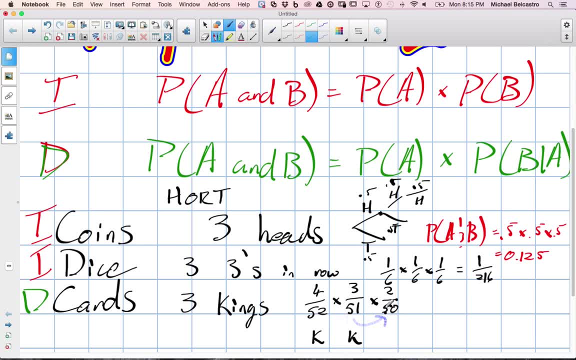 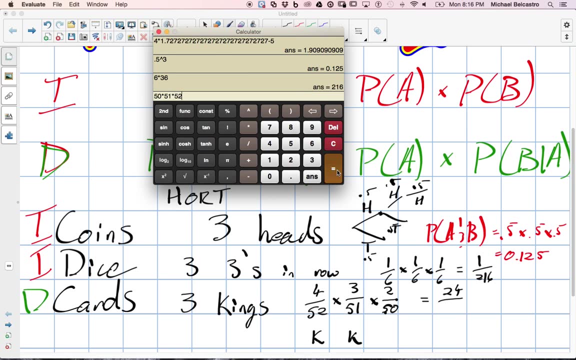 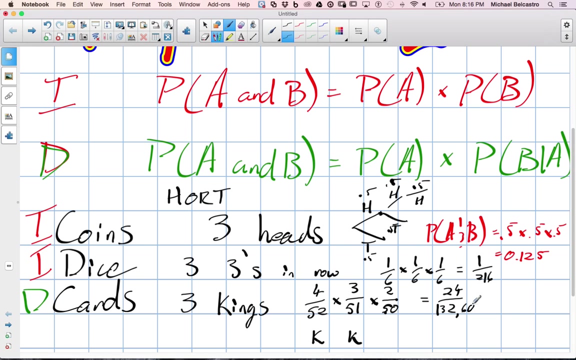 dependent. this is a dependent event. now, um, we'll quickly calculate this here. uh, four by three is 24 in and we'll do 50, 50 times 51 times 52, 132 600, so 132 600. so the probability is super rare. 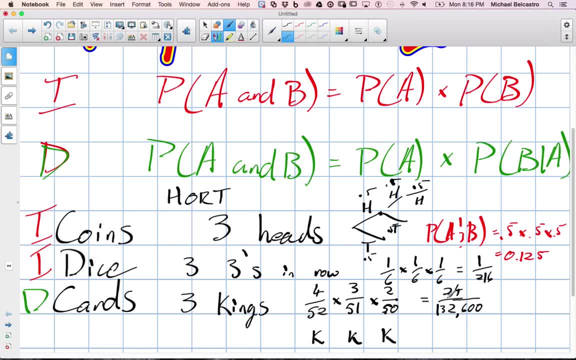 that you get three kings in a row here. okay, so that's how you calculate you, just obviously the probability of the next event. so that would be event b- is um. get a switch changed. given a right, i could make cards independent if i draw the king and then so imagine we have our deck of cards and